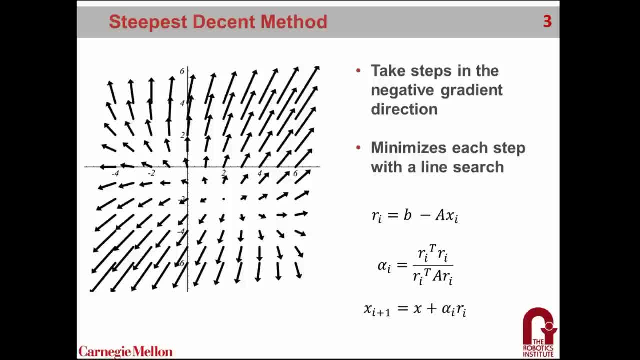 background. we're reviewing the steepest descent method, which is sort of a precursor optimization algorithm. It's called the Conjugant Gradient and it's a pretty simple and effective method. It starts by taking some guess it of x and then finding the gradient at that point. So we saw from. 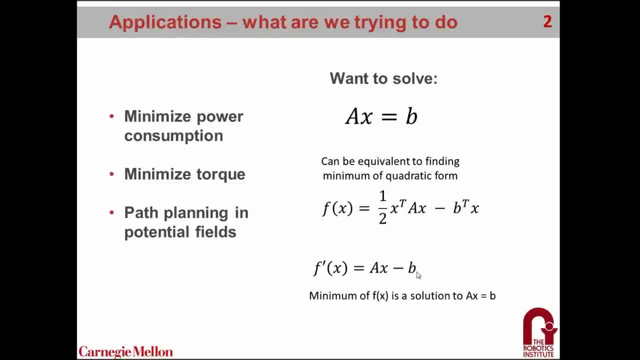 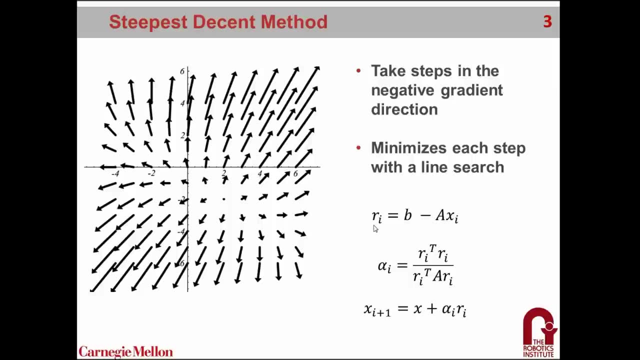 the previous slide that the derivative of the quadratic function is ax minus b, and so the negative of that is just b minus ax, and we'll call that the residual r, which is also the gradient, And that's the vector pointing in the direction of steepest descent. 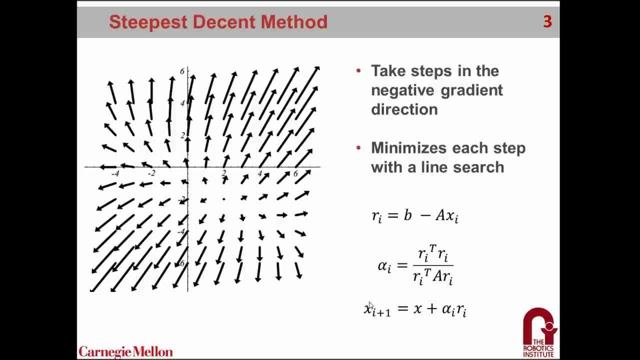 So we're going to call that the residual r, which is also the gradient, And that's the vector pointing in the direction of steepest descent. So all we do to update our new estimating of the solution x is move along the direction. 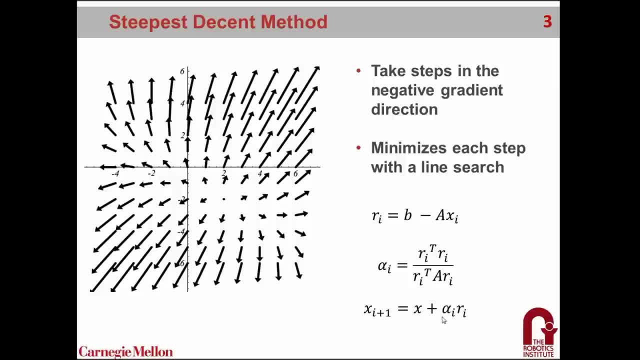 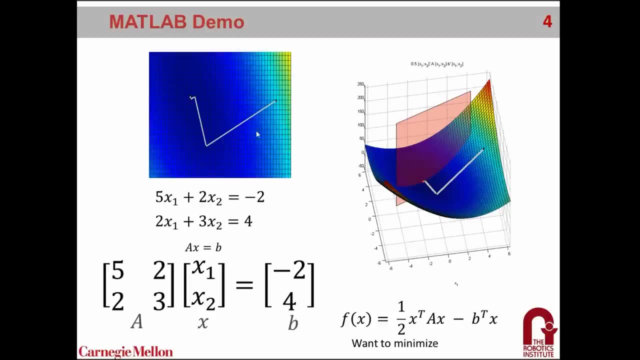 of the steepest descent r by amount, alpha. And alpha is a way of optimizing our movement along this direction in a line search. So we'll take a look at a MATLAB example of this. Here we have two equations, 5x1 plus. 2x1 plus 5x2, which is equal to the Evan's equation. So we're going to take a look at a MATLAB example of this. Here we have two equations: 5x1 plus 2x2, which is equal. 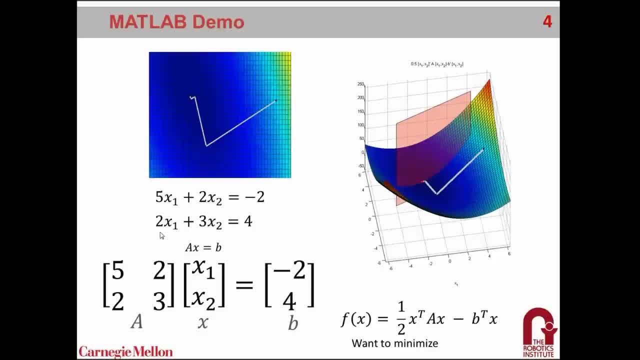 to the Eva equation. So here we have two equations: 5x1 plus 2x2, which is equal to the Evan's equation: 2x2 equals minus 2, and 2x1 plus 3x2 equals 4.. 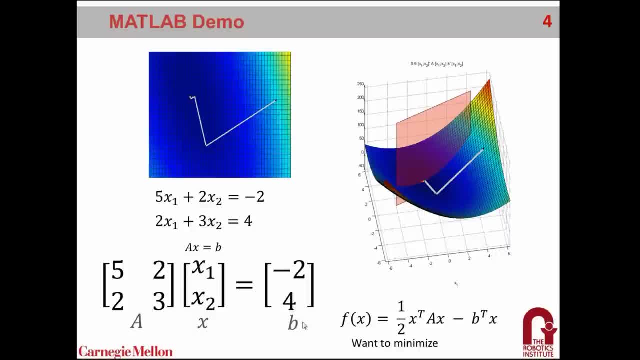 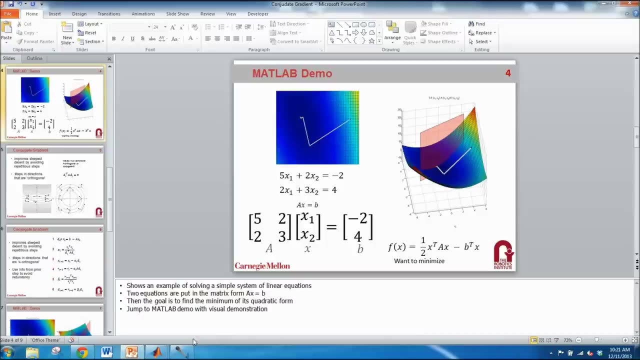 So this system of two equations can be written in the form ax equals b in this matrix form here, And so the goal we want to do is find a solution to this problem by minimizing its quadratic form shown here. So let's skip over to MATLAB and run a script. 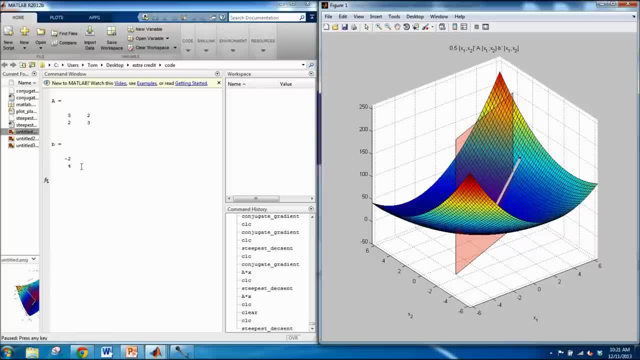 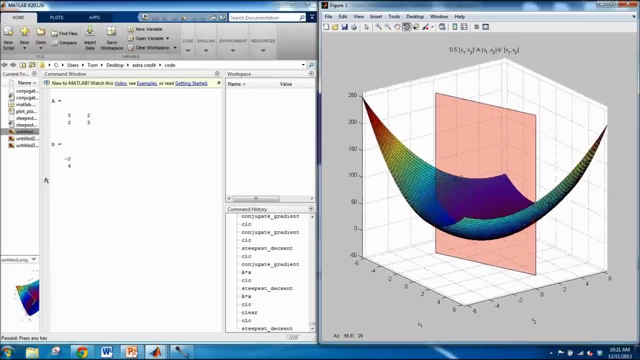 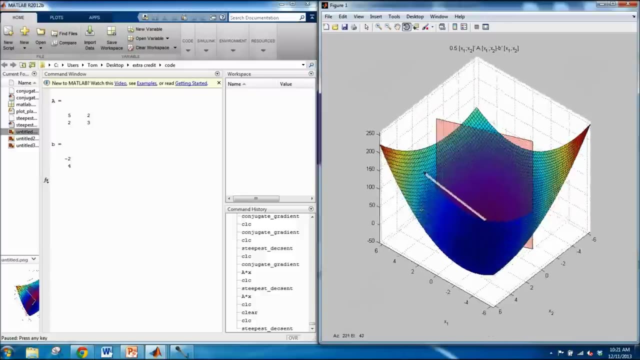 So, as I mentioned, we have our matrix defined here and our b vector defined here, And this plot here shows the quadratic function which is what we want to find the minimum of, to find the solution to our linear system of equations. So this black dot here is our initial guess of where the minimum would be. 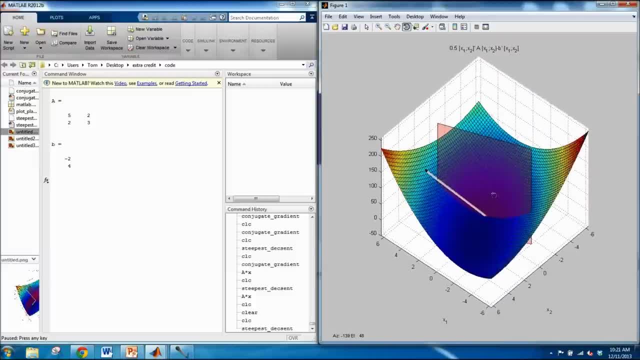 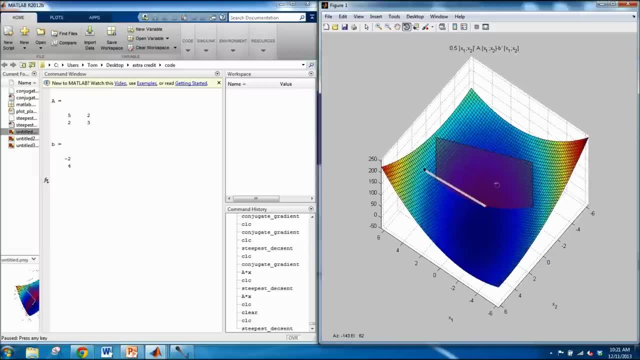 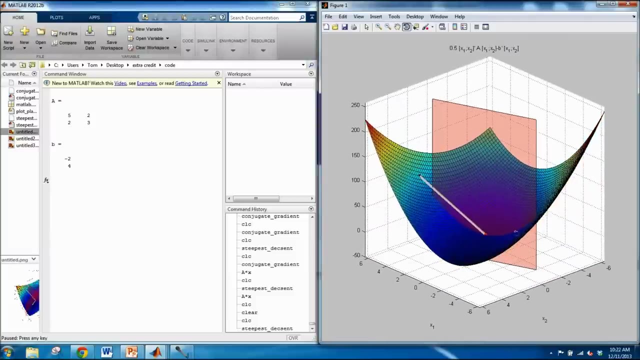 It's pretty arbitrary. it doesn't matter where you start, And so then you take the gradient Or direction of steepest descent at this point and do a line minimization along that direction, So you can see. that's where this plane intersects the function we're trying to minimize. 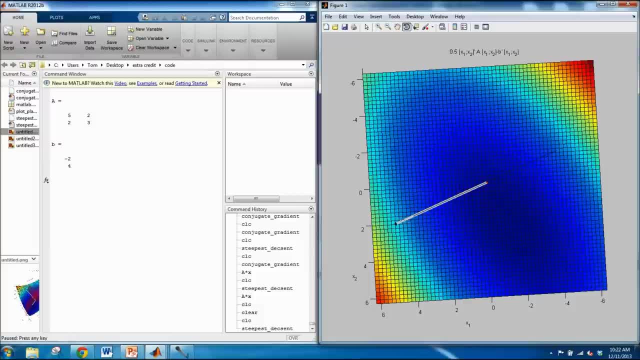 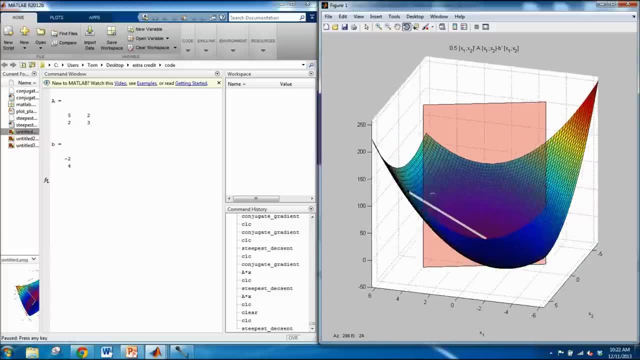 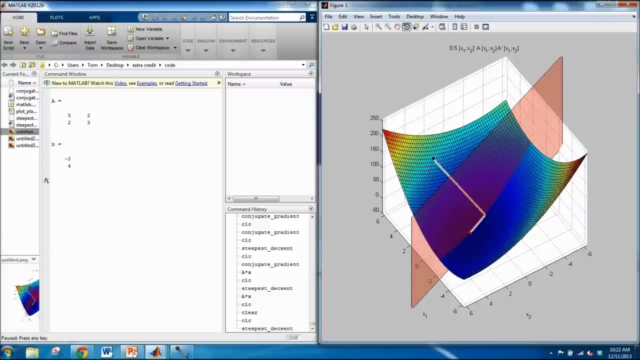 From the top view you can see we're trying to find a minimum along this line, which is bound to be the red point right here. So now we use this as our new guess of x. So we calculate this, Calculate the gradient again and get a new direction of steepest descent shown by this plane which points us in a new direction. 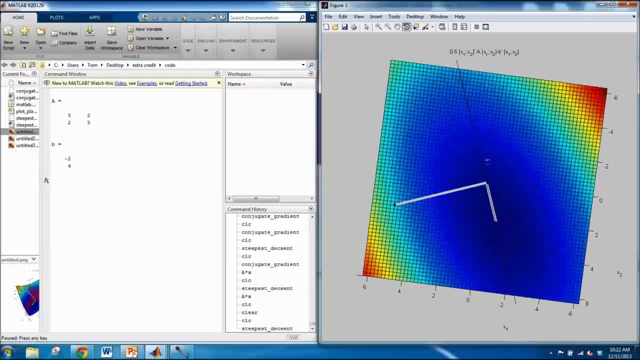 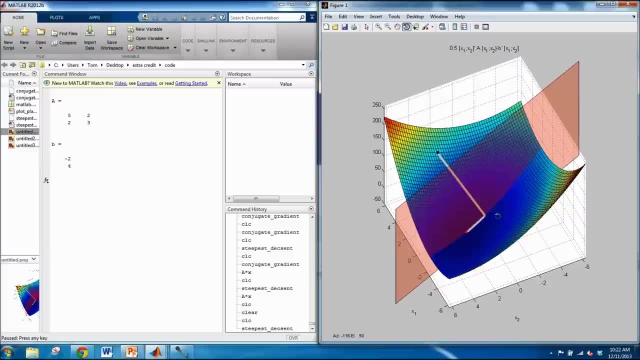 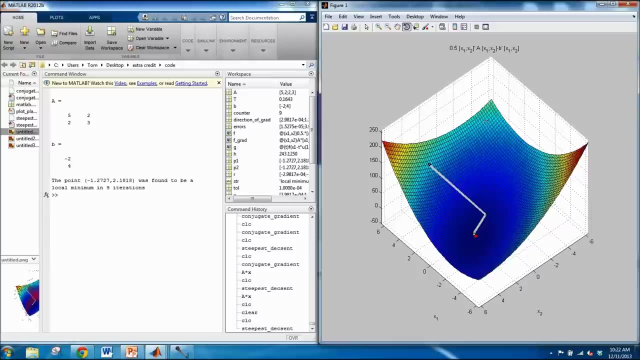 And again we do a line optimization search along this intersection and find that the minimum was here. So this is repeated to some convergence criteria And eventually we see that it found a point minus 1.27 and 2.18.. It's found to be a local minimum at 9 iterations. 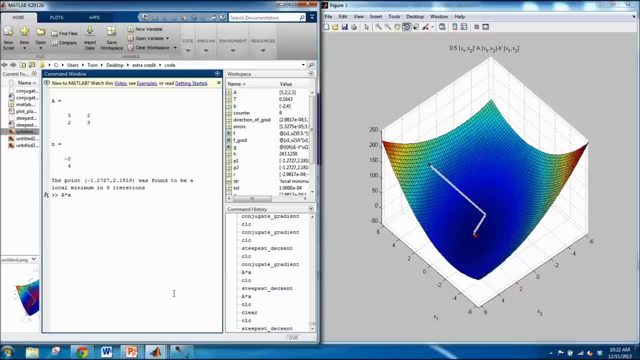 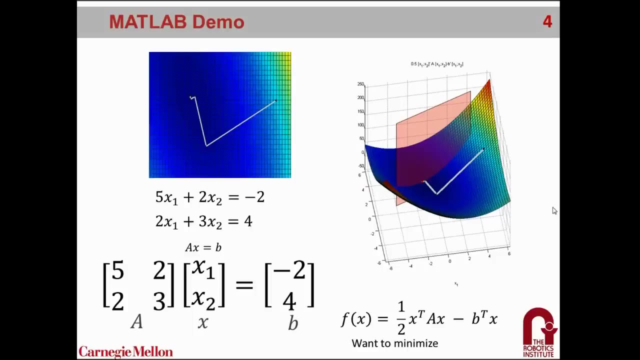 And to check that we can do our A matrix times the x that it just calculated And see that we get our B vector back minus 2 and 4, which is what we want. So this is not a bad method. It got us there in 9 iterations in this example. 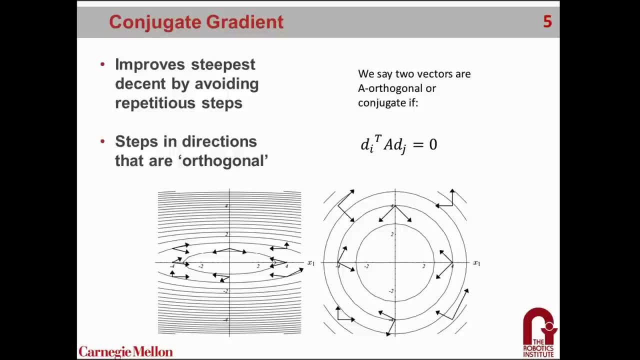 But country and gradient asks: can we do better than steepest descent? And the answer is yes by taking steps that are orthogonal or more specifically, a-orthogonal. So we define two vectors to be a-orthogonal. if di transpose a dj equals 0,. 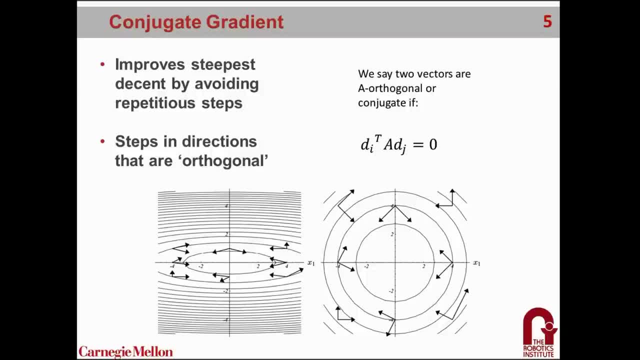 which is a little bit abstract, but you can visualize it By these plots. So this is a contour plot with pairs of vectors that are a-orthogonal And if you can imagine that this sheet of paper is stretchable, so you can warp it and stretch it in different directions. 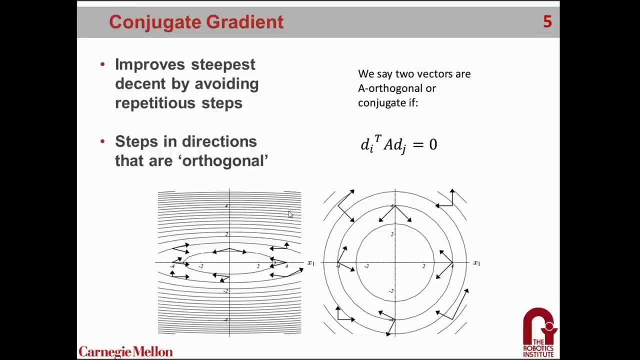 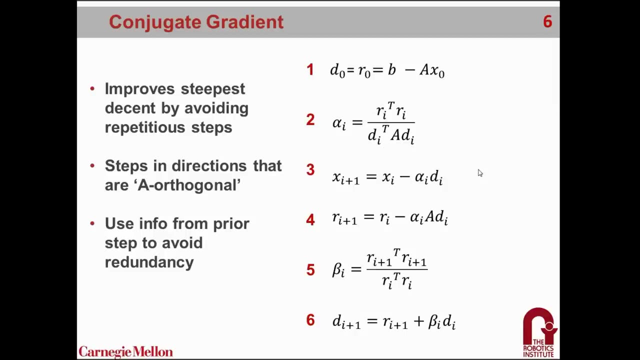 then you could imagine stretching it out so that the contours are circles, And that results in what you see here, where now the vectors are orthogonal in the conventional sense, which is the dot product is 0, and they are perpendicular. So the result of this method is that new residuals are orthogonal to all previous residuals and search directions. 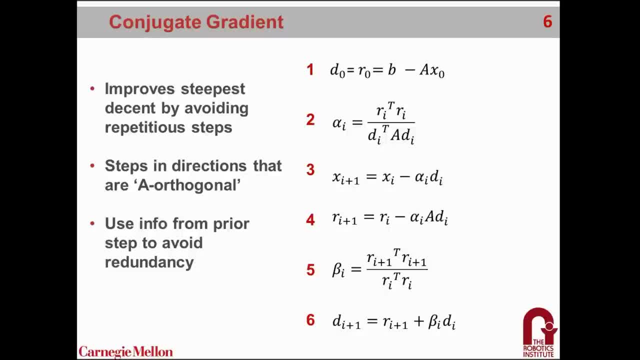 And new search directions are constructed from the residuals to be a-orthogonal to all previous residuals and search directions. So, without going into too much detail, this is the resulting algorithm that accomplishes that. It starts in the same way that steepest descent does. 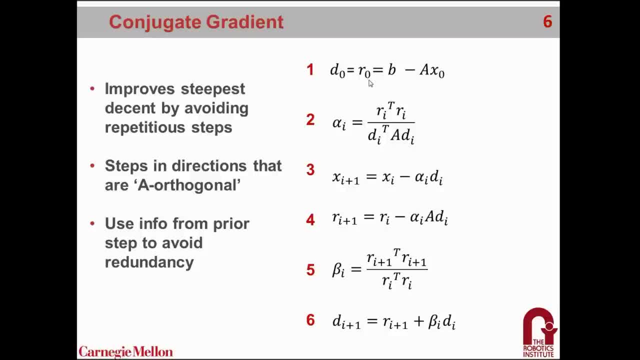 by initializing the d and residual r vectors to just be the negative gradient And then the rest. these five iterative steps, repeat at each iteration And you can see they're really not too different from steepest descent. And you can see they're really not too different from steepest descent. 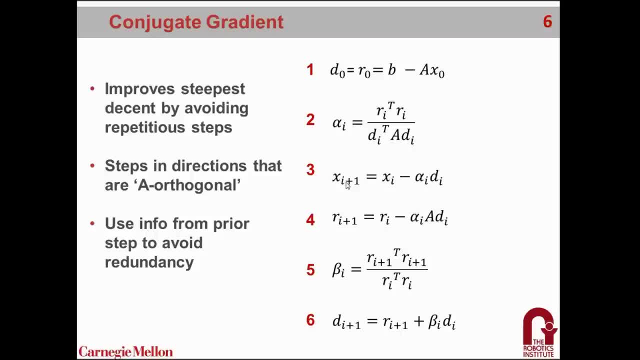 And you can see they're really not too different from steepest descent. Instead of updating x along the direction of the steepest descent r, it's now along the direction of d, which is constructed to be a-orthogonal from the residuals. 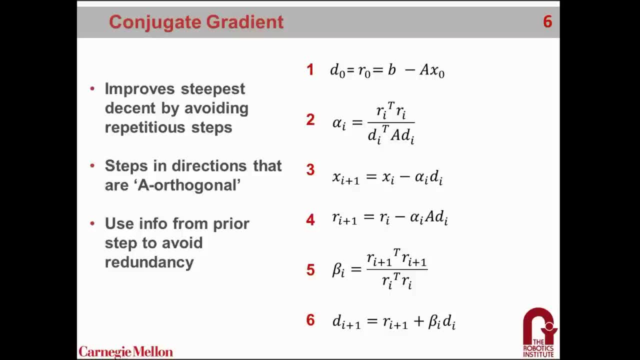 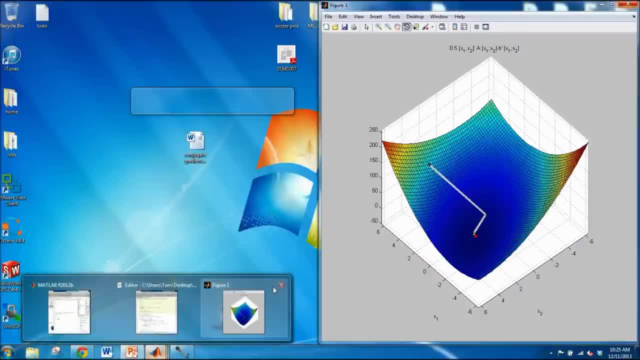 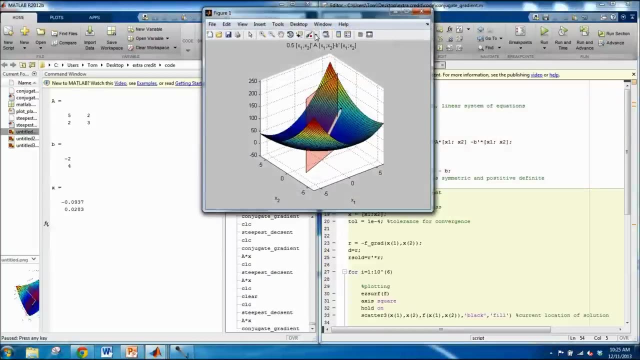 So this turns out to be a pretty powerful tool. So this turns out to be a pretty powerful tool. And optimization techniques. We'll go back to the same MATLAB demo And now run conjugate gradient. And now run conjugate gradient. So we have the same problem here. 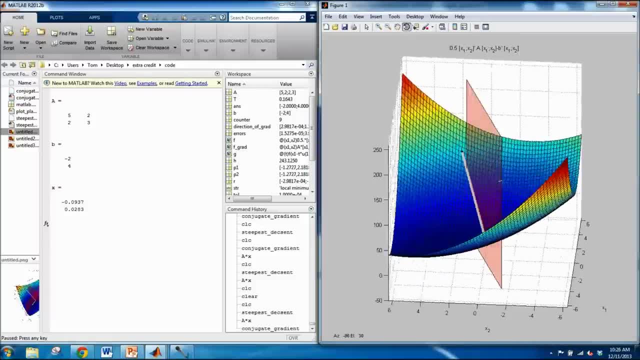 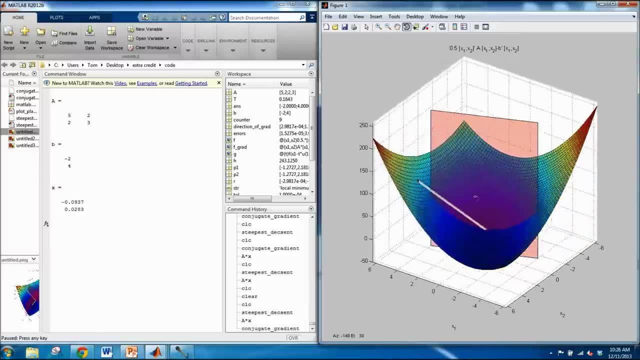 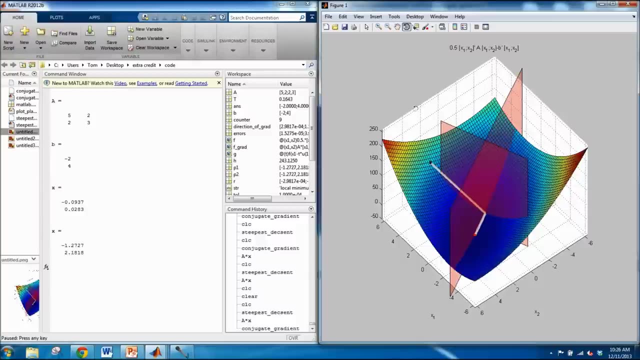 we have the same initial guess point up here and you can see the first step looks about the same. And you can see the first step looks about the same. But what's important is, the second step gets us to the same solution which you can see is much quicker than what Cephas Ascent did. 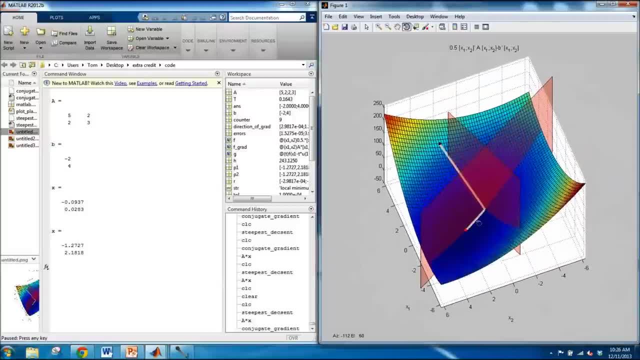 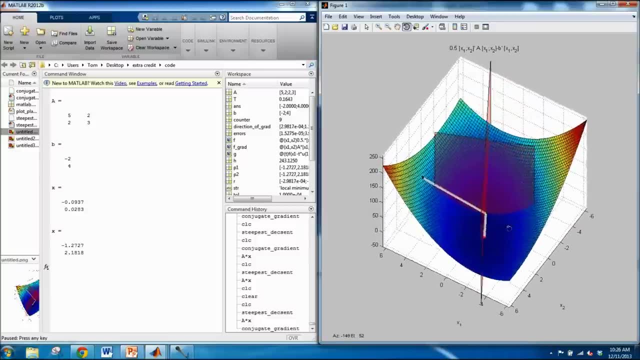 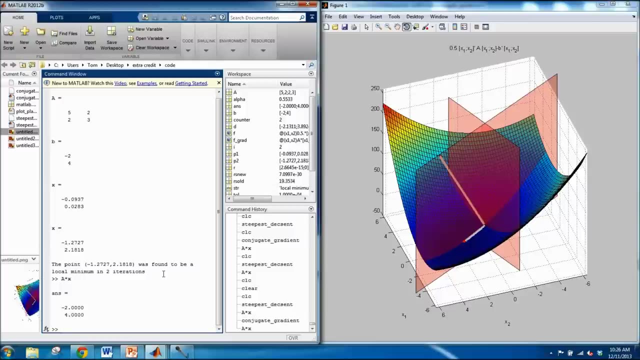 And this is because it's taking steps that are a-orthogonal, so that future steps never undo or redo optimization that the previous step did, making it much more efficient. And our solution again is the same, and it gets us to our B vector.